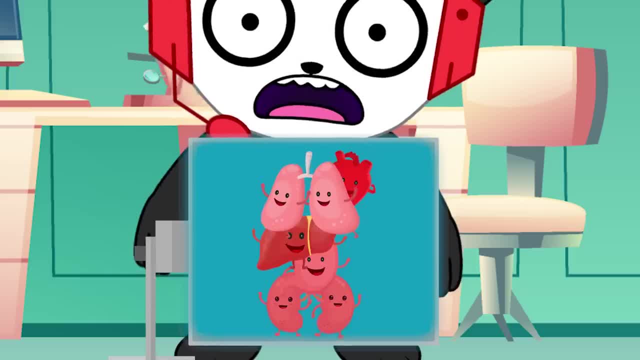 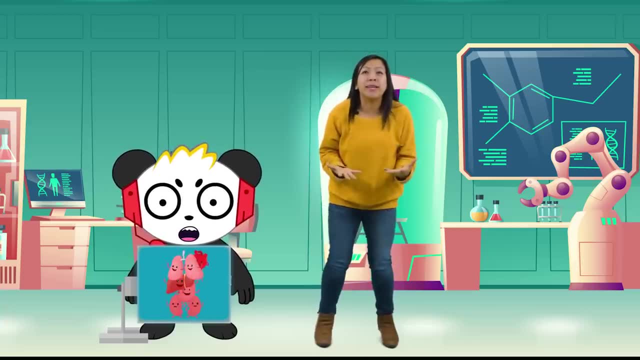 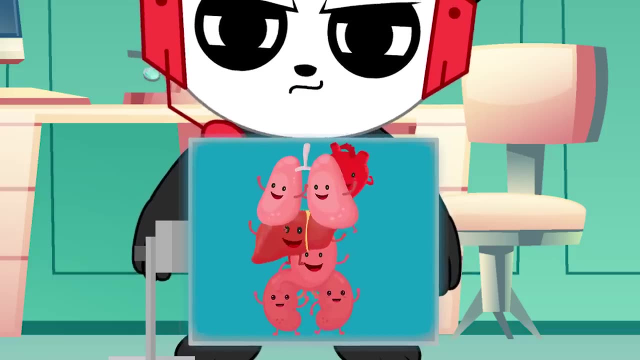 I was trapped in a time machine. Whoa, I can see all my organs. Yes, It worked. Okay, let's point out what we can see. Combo, do you know which organs are which? Um, I can see a heart and something that looks like it's eating my stomach. 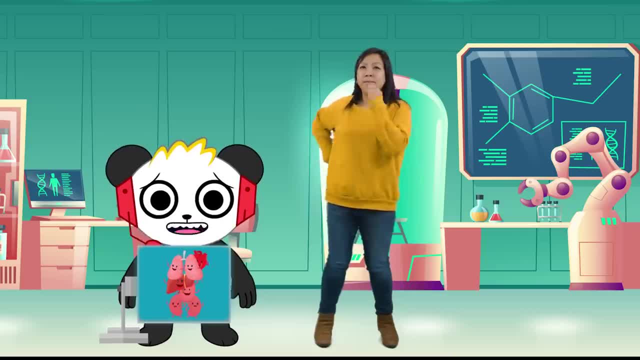 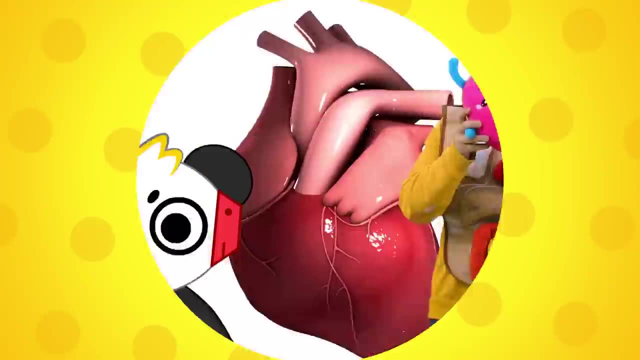 And two giant beans. I don't remember eating giant beans, though. Okay, how about we try this? We can go through each organ one at a time. Well, okay, good, That sounds a lot less overwhelming. Okay, let's start with the heart. Do you know what the heart does? Combo? 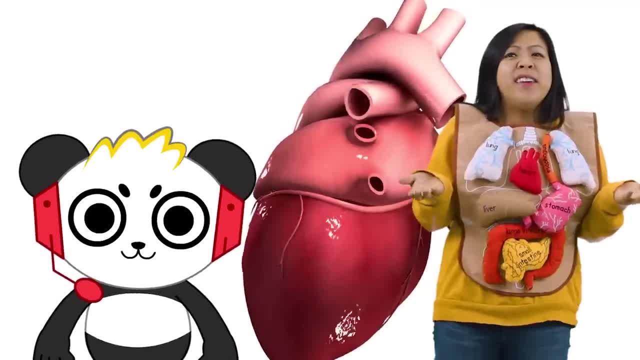 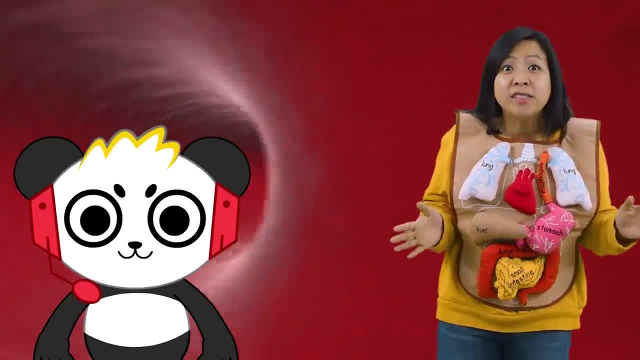 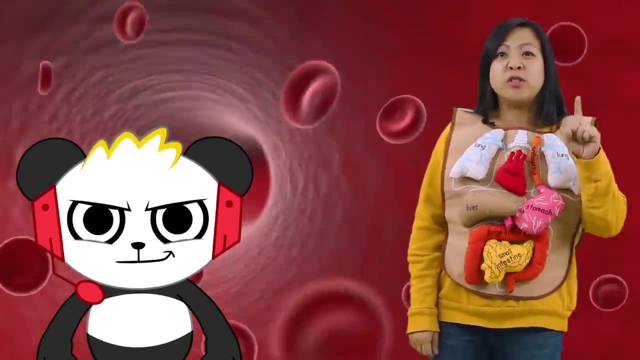 I know that one. It goes thump-thump, right. Well, yeah, So thumps are rhythmic contractions that pump blood into all parts of your body. Combo Bunga, I was right, But did you know there's two sides to the heart? 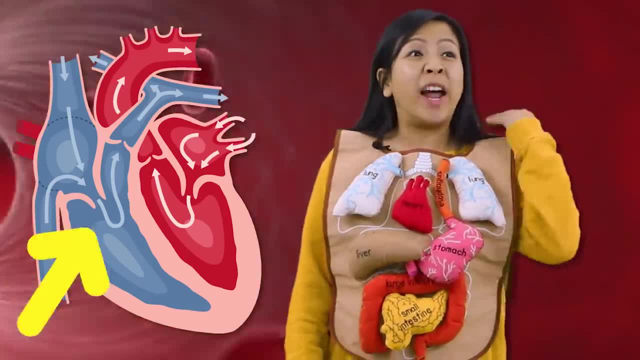 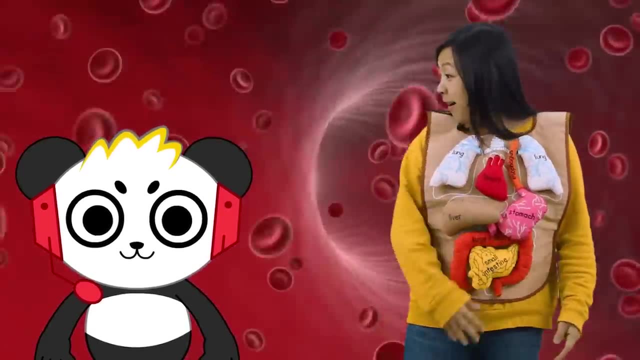 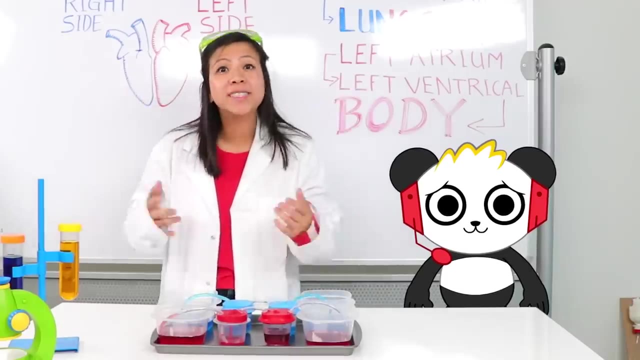 No, I didn't. Yup, there's a right side and there's a left side. Come on, I'll show you in an experiment, Combo, Okay, Hey, this isn't a heart, I know, but this will show us how both sides of the heart work. 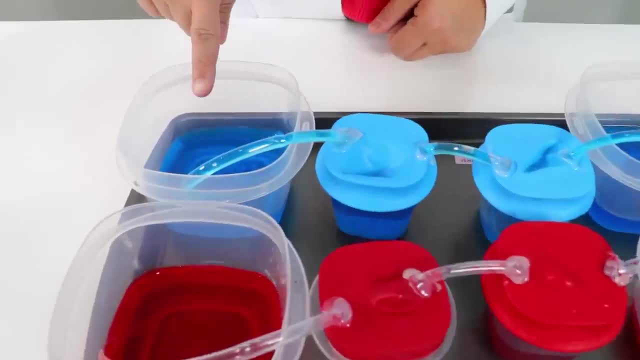 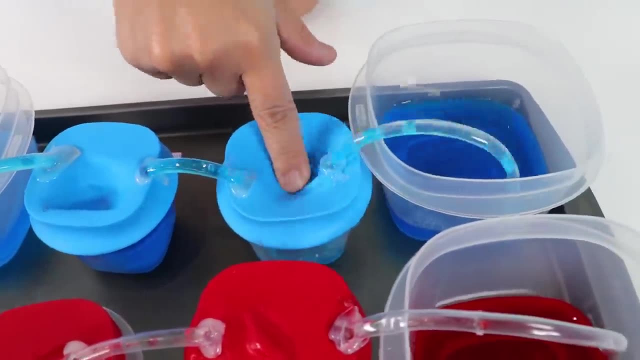 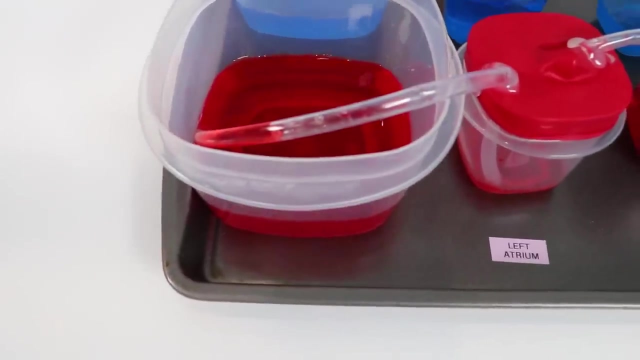 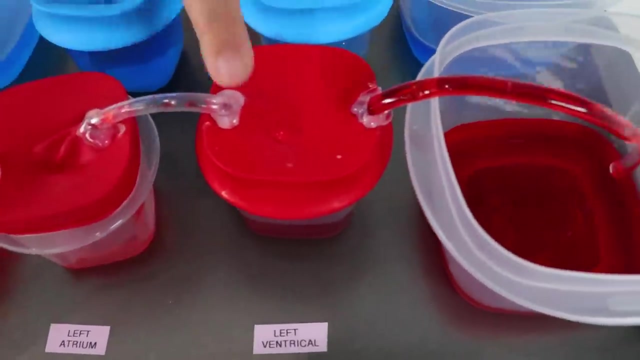 So we have all this oxygen-empty blood and it pumps from the right atrium to the right ventricle and into the lungs. The lungs gives the blood oxygen and turns the blood red. Now that we have this red blood, it gets pumped from the lungs into the left atrium. 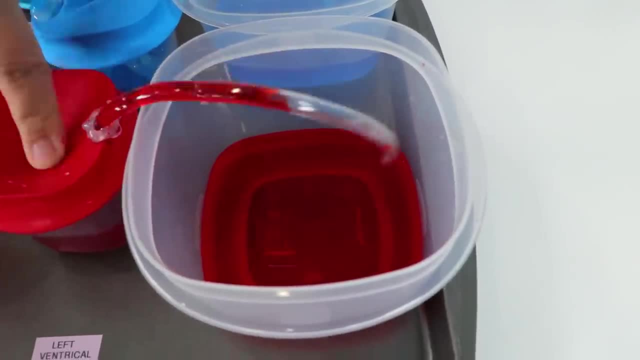 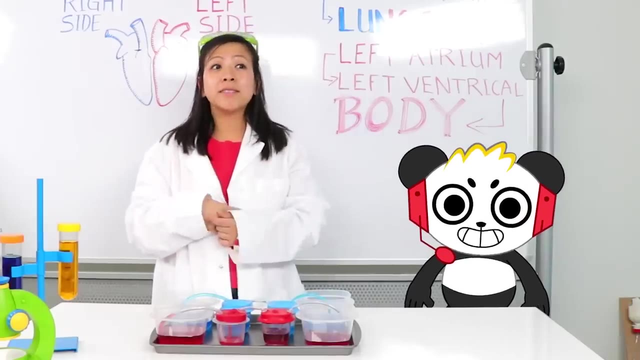 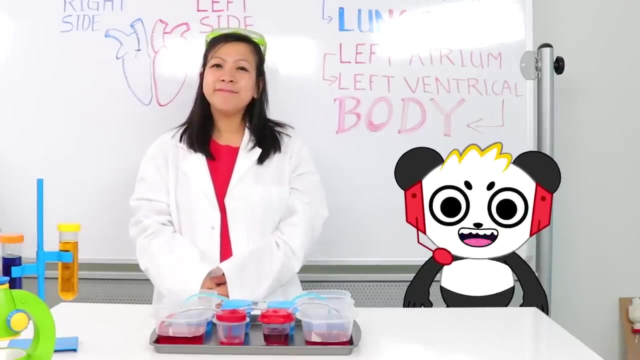 then it goes to the left ventricle and finally out through the rest of the body. Whoa, So it pumps through one side, gets oxygen, then takes the oxygen everywhere in the body. Yup, So I have one question: Where exactly does the lungs get this oxygen from? 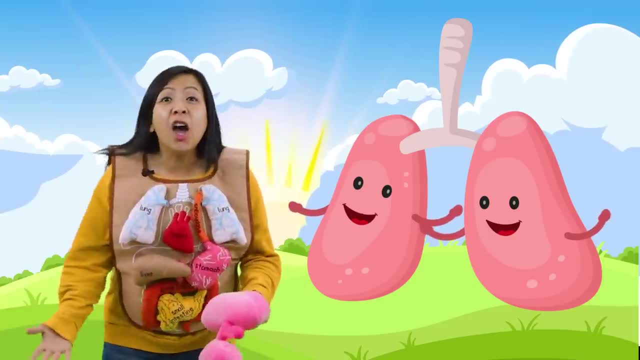 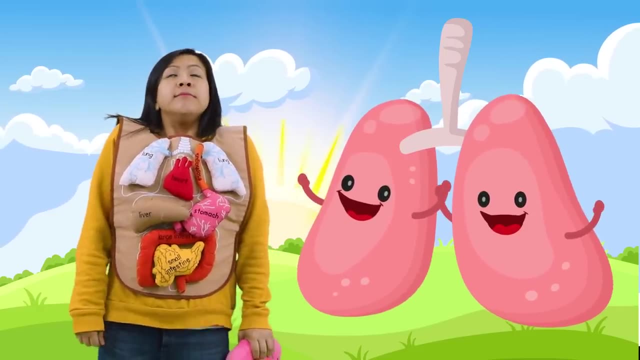 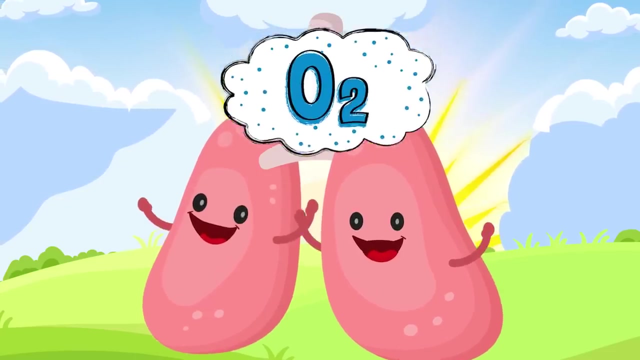 Good question, Combo. I'll show you, Come on. So when you breathe, you are using your lungs: Inhale, Exhale. It's the lungs' job to take the oxygen in your body and remove carbon dioxide from your body. 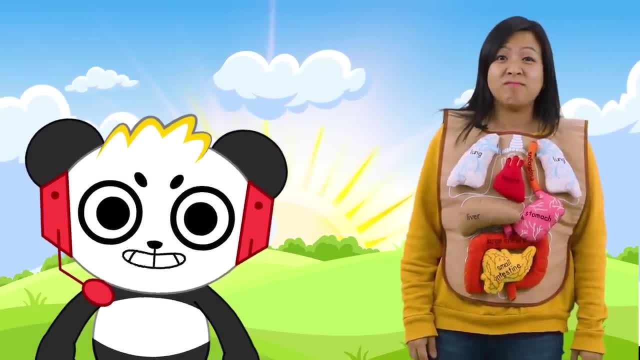 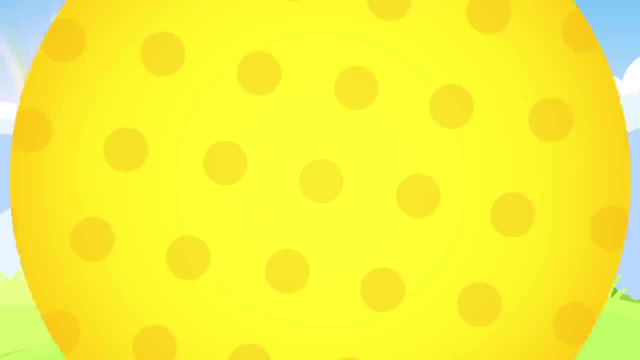 So that's what happens when we breathe. I get it now, That's right, And I know just the experiment for this. Let's go. Combo, Whoa, Is that supposed to be our lungs? Yup, This bottle is like our body. 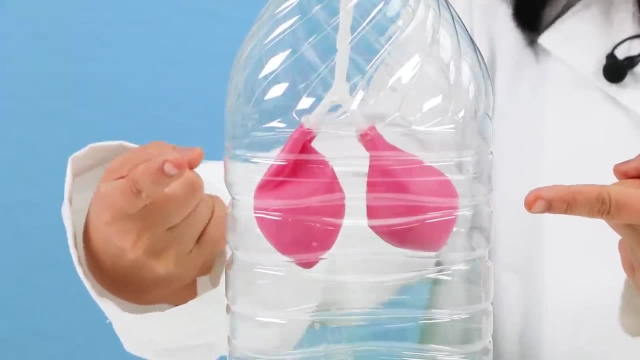 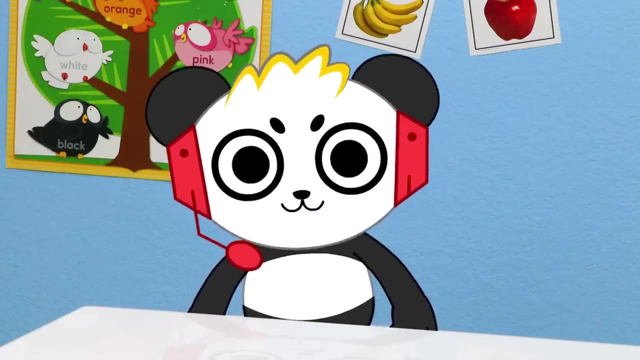 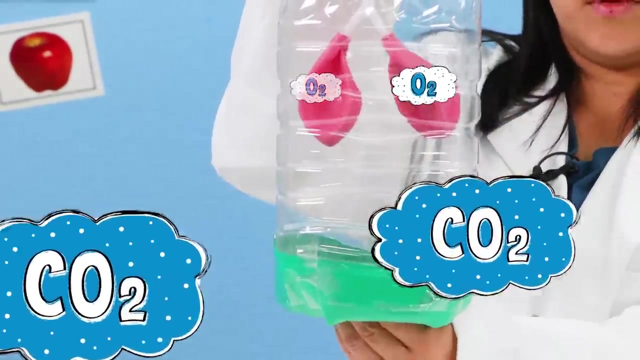 and the balloons inside is like our lungs, So we'll be able to see the lungs expand with oxygen and then shrink when releasing carbon dioxide. Yeah, see, Look, Do you see how the airs are going into the lungs? That's so cool. 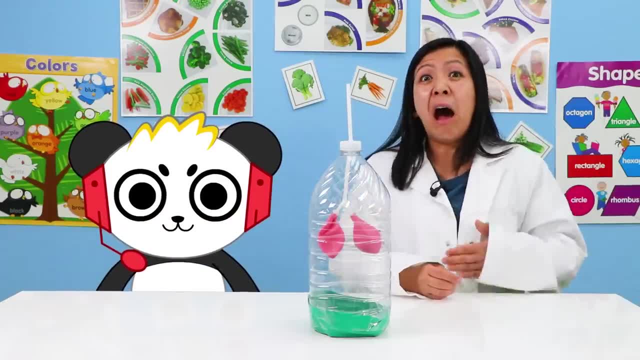 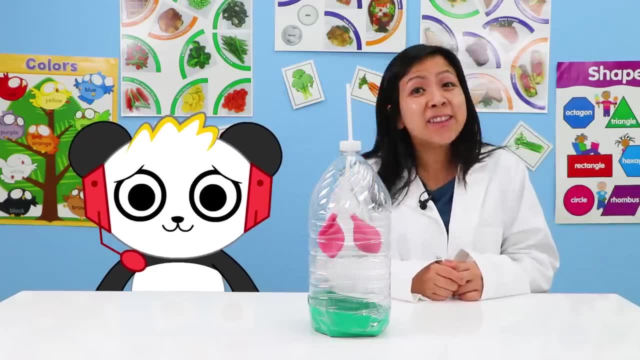 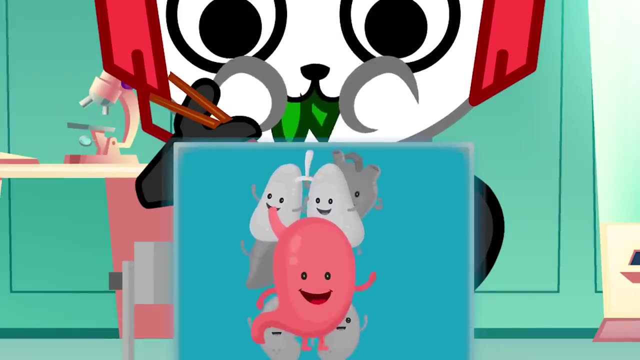 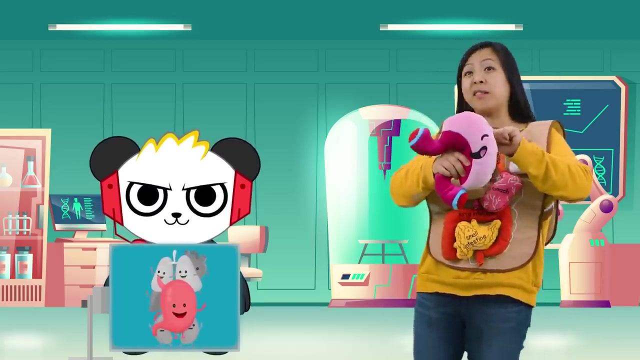 Uh-oh, Sounds like someone is hungry. Yeah, I think it's time for a snack. Okay, Combo, We can eat and learn As long as I get to eat. Mmm, That was delicious. Okay, are you ready to learn about the stomach now? 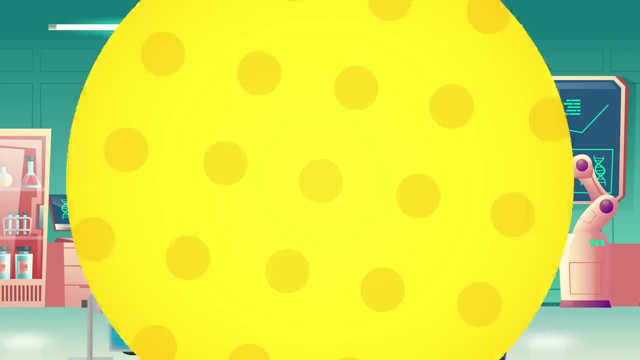 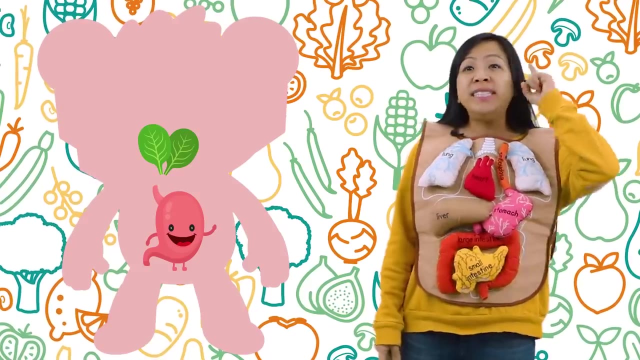 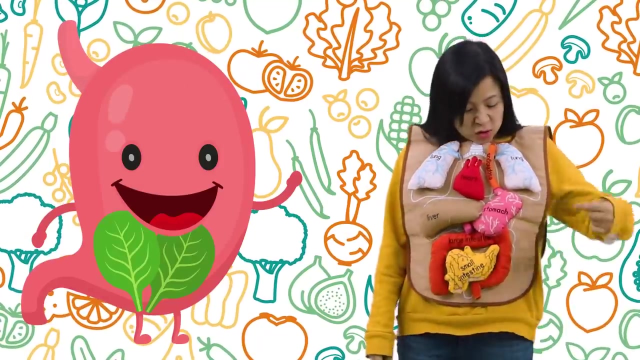 Well, mine is full, so learn away. Okay, so when Combo ate his food, the food went from his mouth down his throat and into his stomach. right Once it gets to the stomach, it is the stomach's job to store the food. 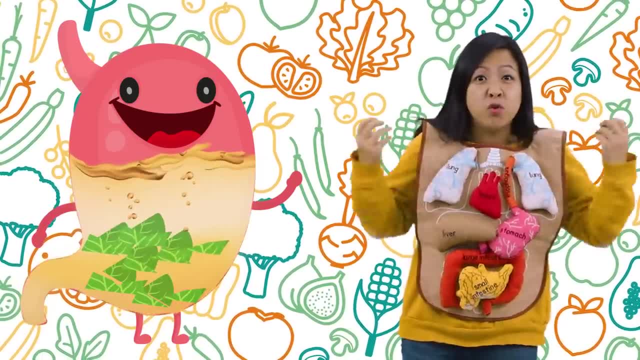 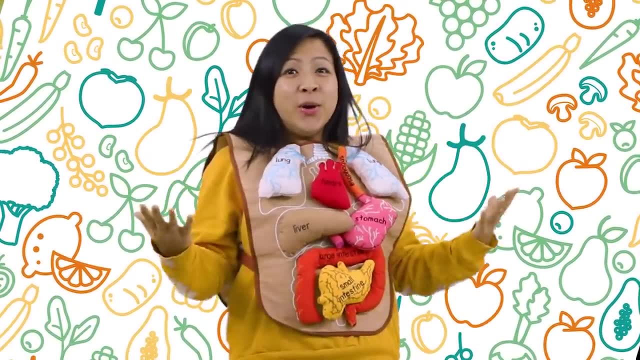 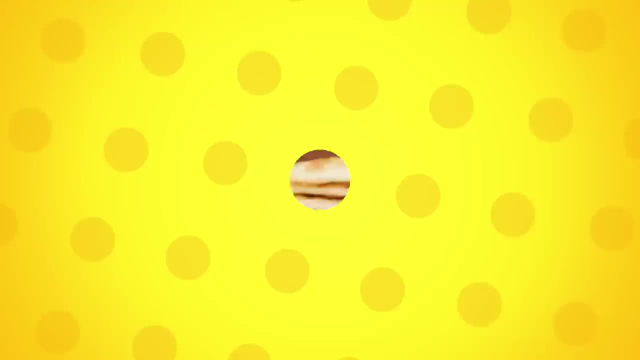 digest the food and then mix the food. How does it do all that? I'm happy you asked, Combo, let's do An experiment. Yeah, That's what I'm going to say. Come on, Yeah, So it looks like we get to snack on some crackers. 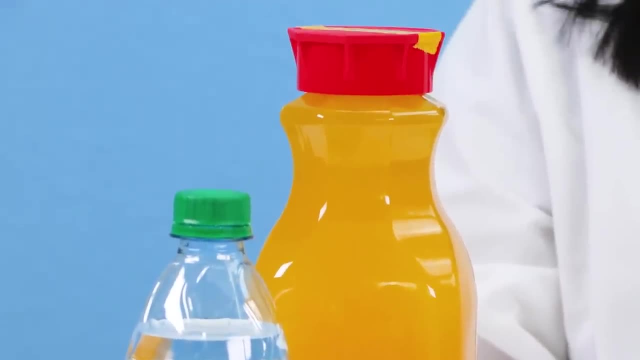 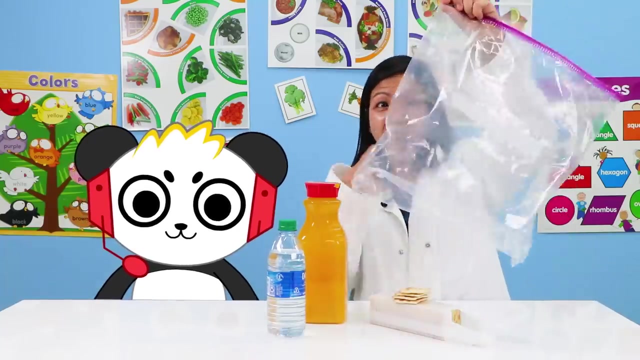 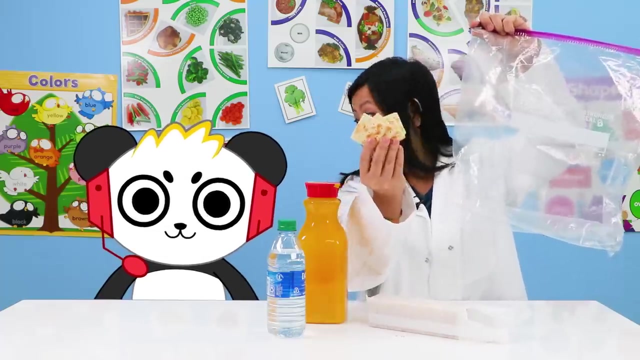 and wash it down with some orange juice. This might be my favorite experiment, yet Not exactly. Combo Aw man. So this bag is like our stomach and let's say, today we eat some crackers. So far, so good. 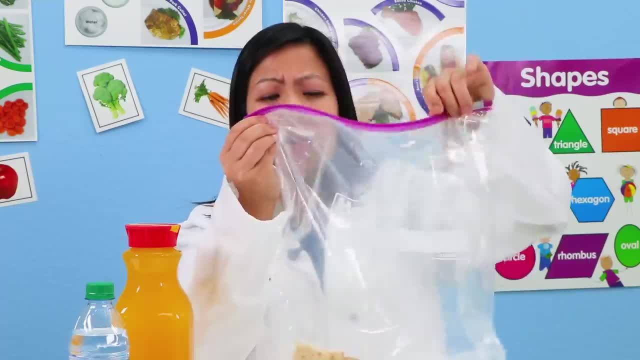 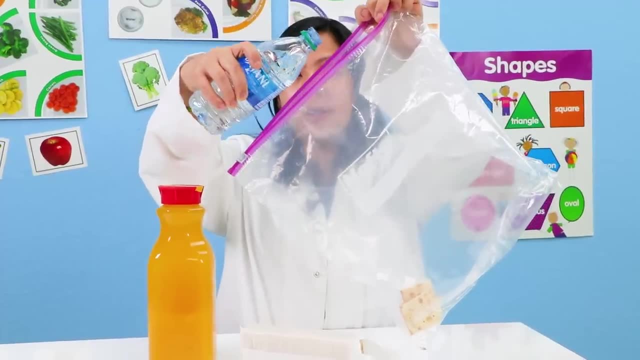 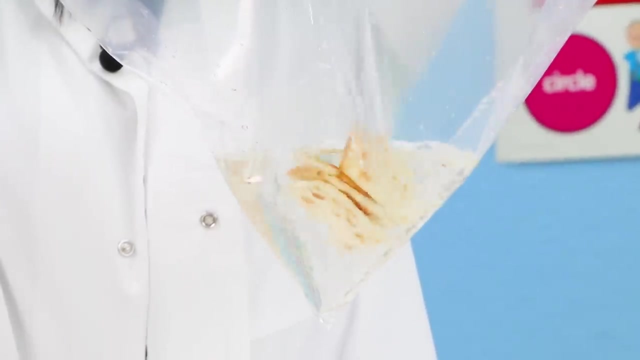 Okay, so you're eating the crackers Now these crackers are kind of salty so we want to wash it down with some water. Here we are drinking some water. It's going into our stomach. It's looking kind of gross in there. 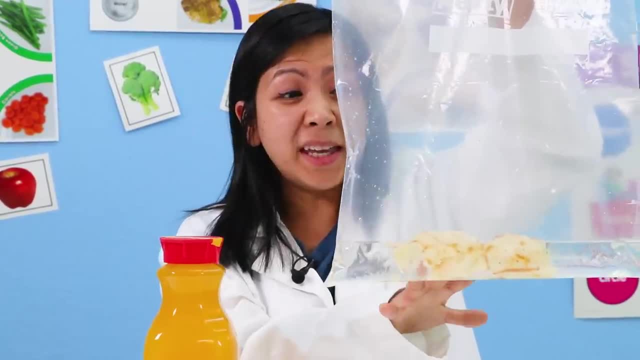 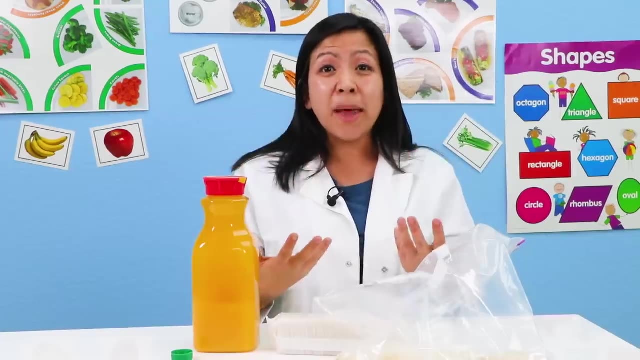 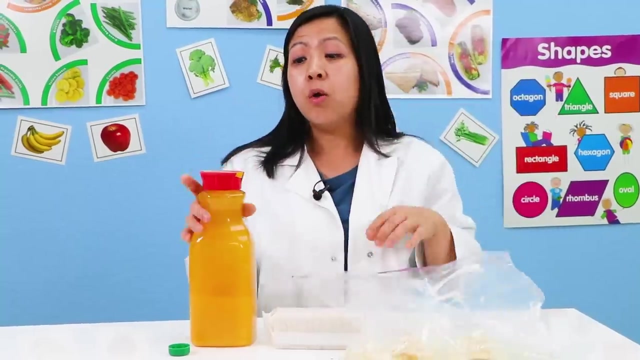 Yes, it does look gross. And once all your food make it into your stomach, your stomach has to digest. it Digest. How does it do that? Our stomach has juice inside called stomach acid that will break down our food. So we will use orange juice to show stomach acid. 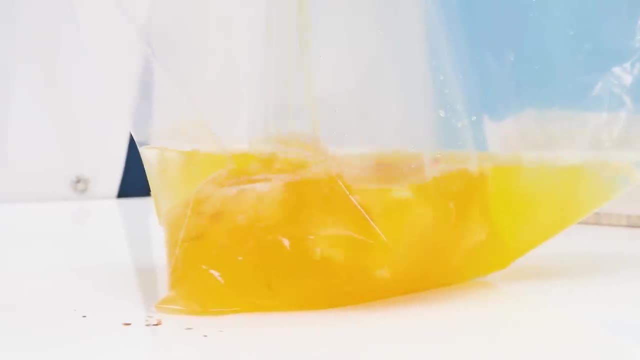 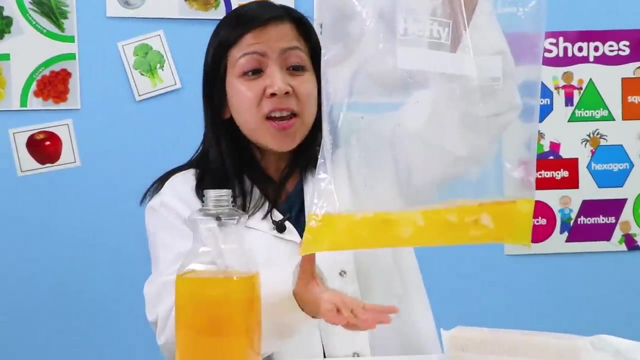 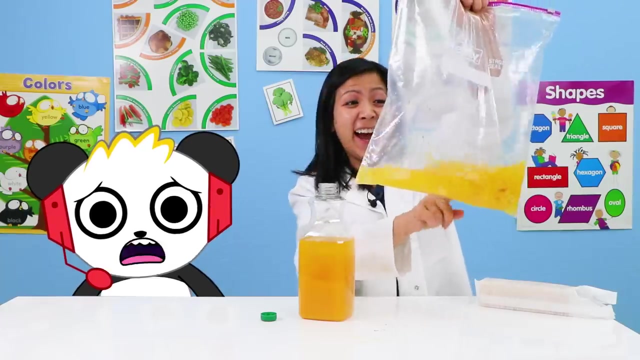 Here's the stomach acid. Ew, Hang in there. We're going to close it and mash it all up, just like how our stomach digests and mix our food together. What do you think? Okay, can we move on to another organ? 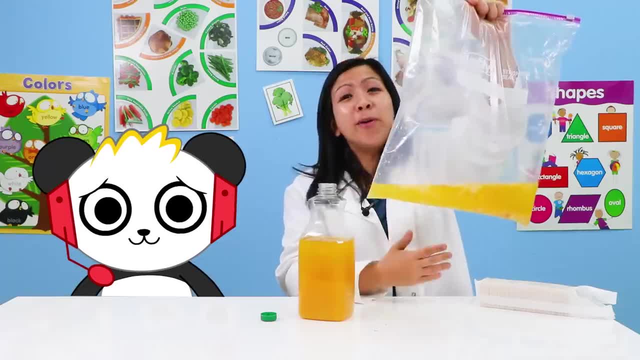 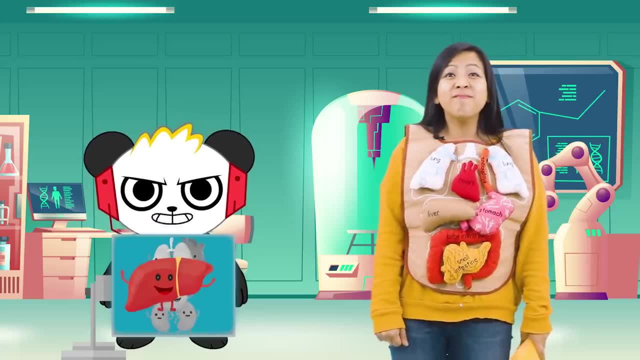 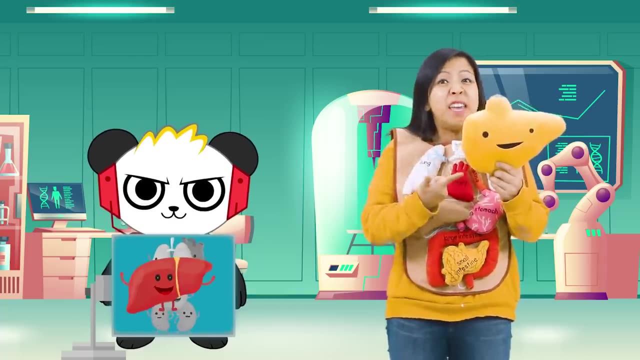 My stomach is getting a little queasy now. Okay, Combo, let's move on to the liver. Okay, so, this liver thing that's bigger than my stomach. what does it do? Your liver cleans your blood. It's the liver's biggest job. 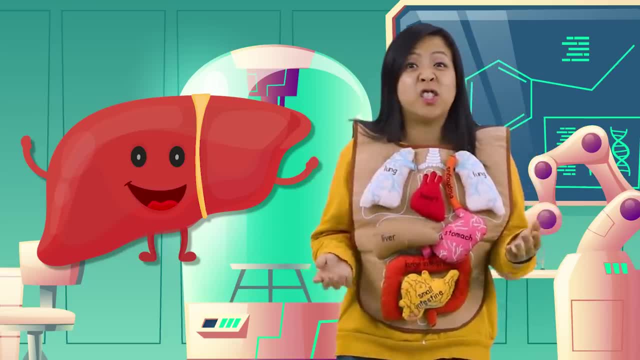 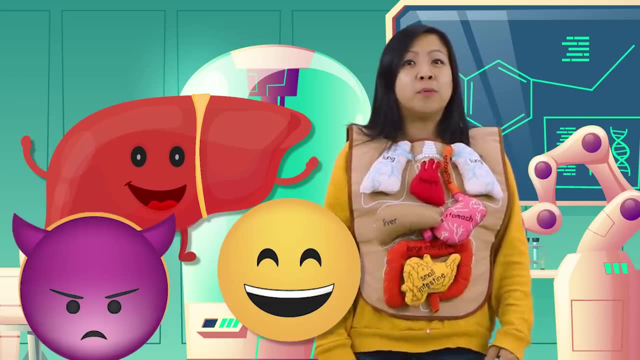 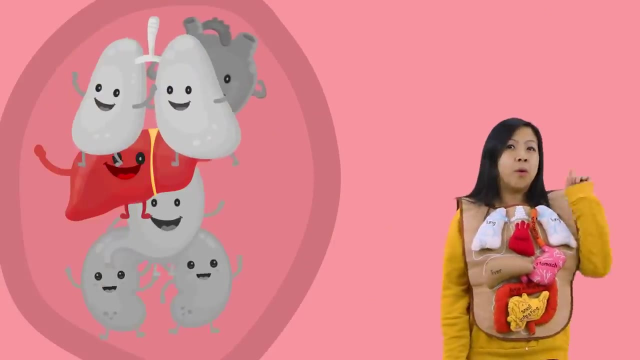 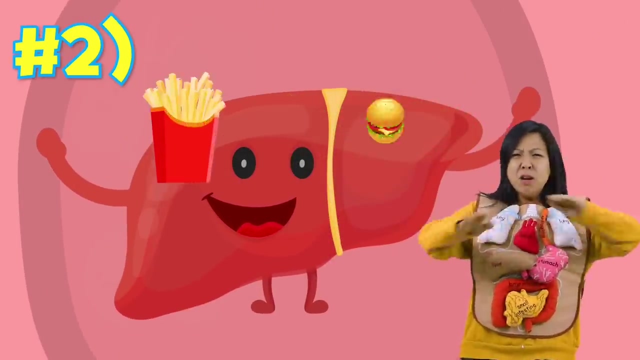 Cleaning blood. Yeah, your liver is smart. It knows what's good and bad for your body. It keeps your blood clean by controlling nutrients in three ways. Number one: it helps us absorb good nutrients. Number two: it removes bad nutrients. 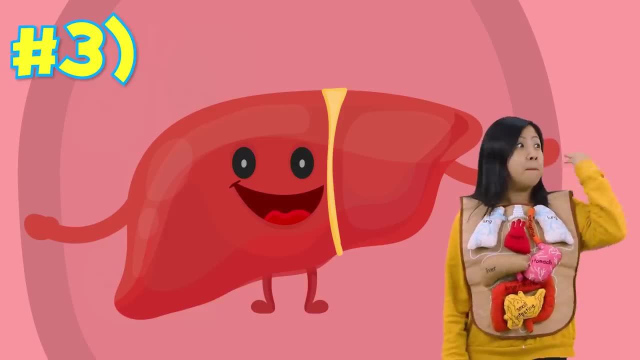 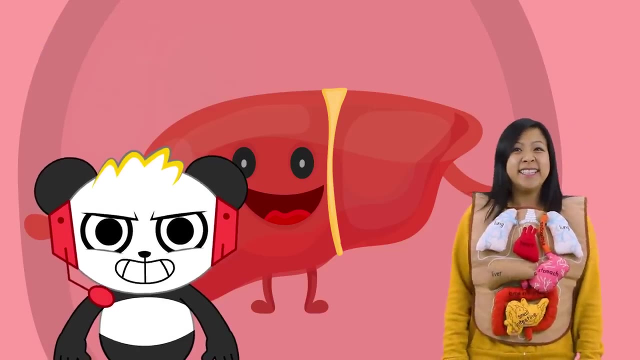 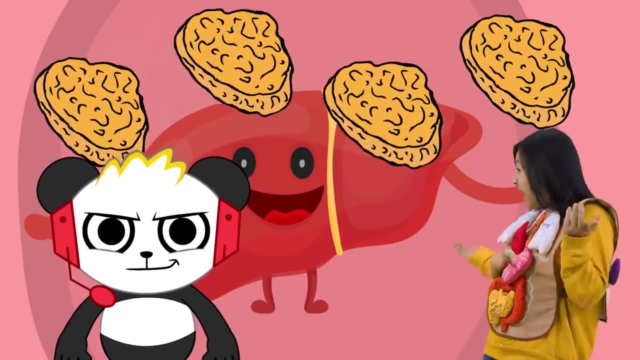 And number three, it can also turn bad nutrients into something that our body can use. So if I eat a bunch of chicken nuggets, If you eat chicken nuggets, your liver will notice that there's protein in it. Combo, you want to try it with a real liver experiment? 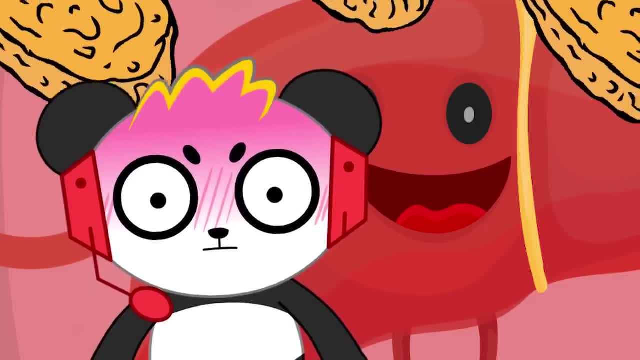 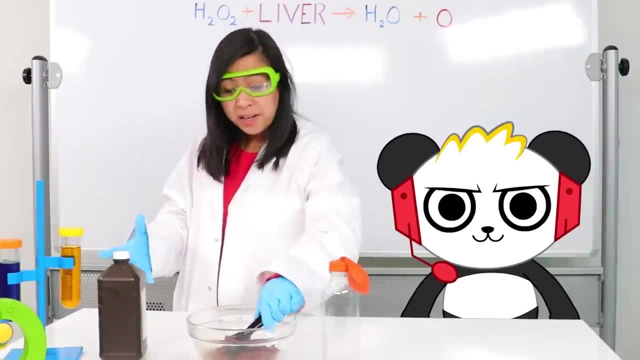 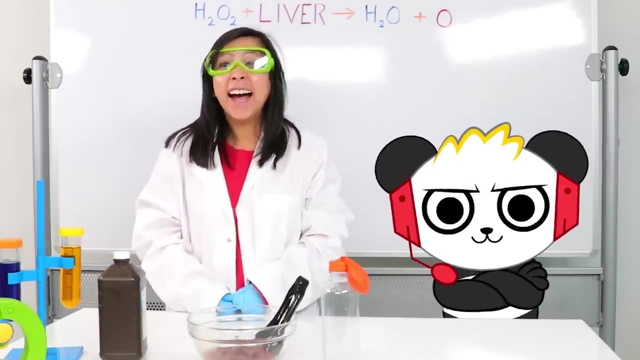 Real liver. Uh sure, My stomach can take another experiment. So we have a liver here. Are you ready to witness the liver in action? I've got to see this. So this is hydrogen peroxide, and people use the hydrogen peroxide to prevent infection. 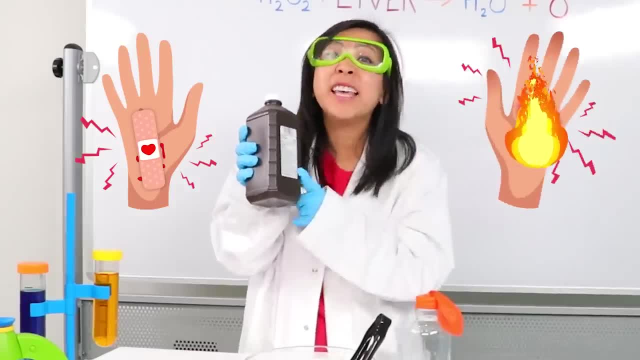 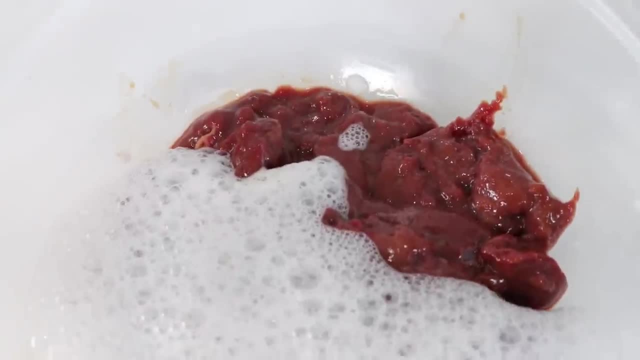 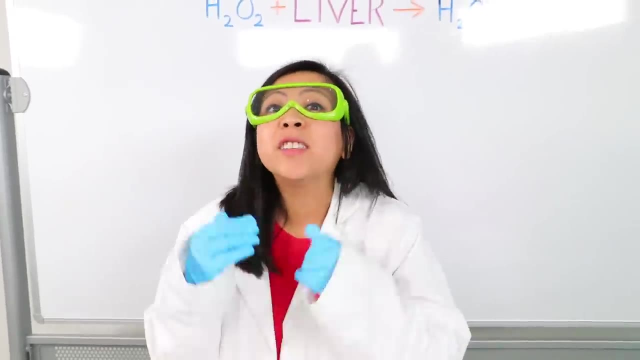 like if you have a minor cut or burn, but this is actually bad for the liver. Watch, Whoa, look at that. What's that? What just happened? What happened to the hydrogen peroxide? So what happened, Combo is the liver split into two parts. 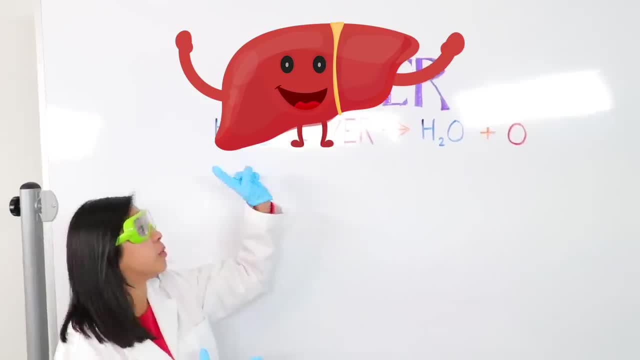 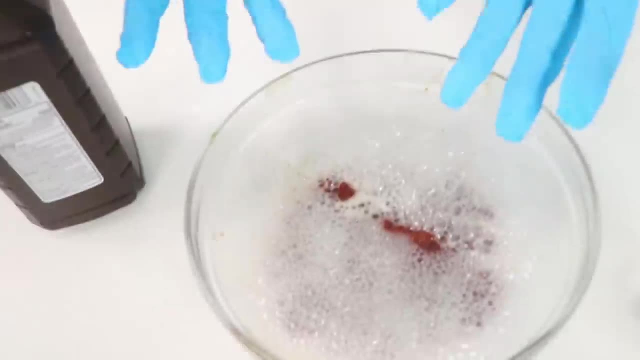 So when you have liver and you pour hydrogen peroxide on it, it converted itself into water and oxygen. So that's why you see the little bubbles there. We put a balloon on top so we can see how much oxygen gets released. 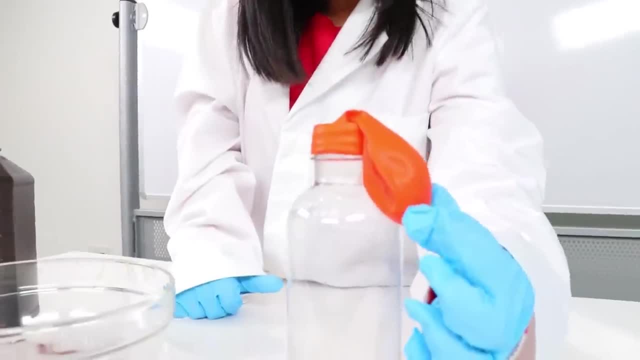 Okay, watch this Combo. So the hydrogen peroxide is in the balloon, We're going to let it go, and then we have a piece of liver on the bottom. Do you guys see that? Let's see what will happen. 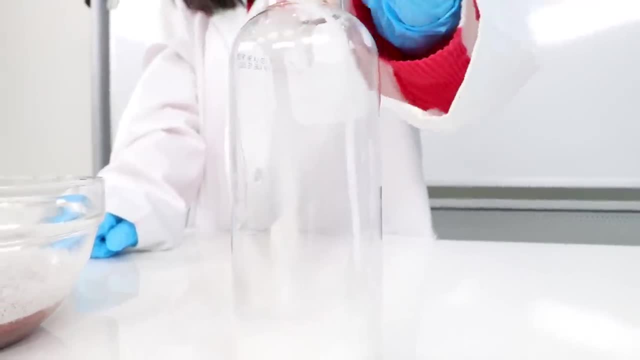 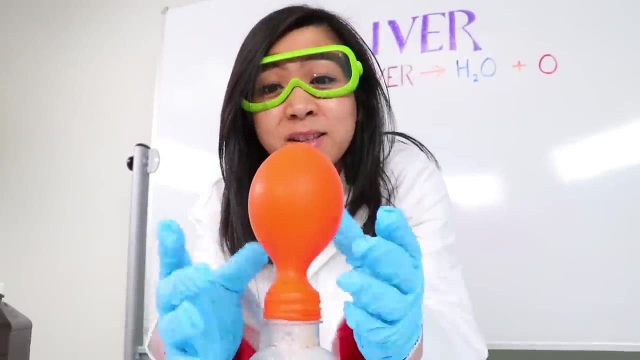 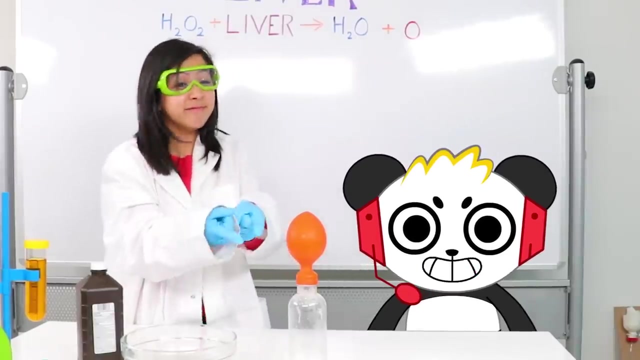 So the liver converted the hydrogen peroxide into water and oxygen, and guess what happened to the balloon? Because oxygen is a gas, and so it inflates the balloon. Look at that, That's cool. Okay, this is cool. Okay, this is cooler than I thought. 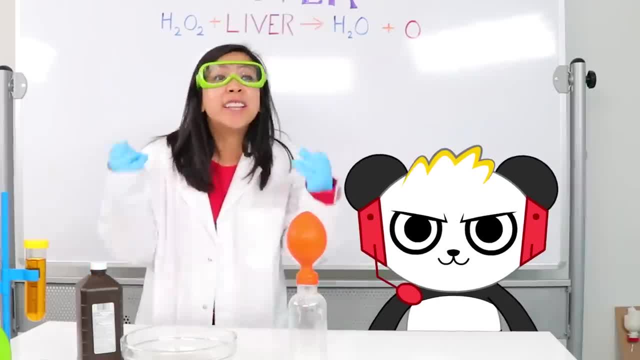 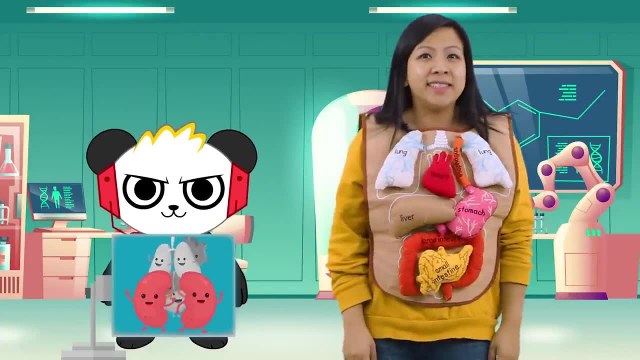 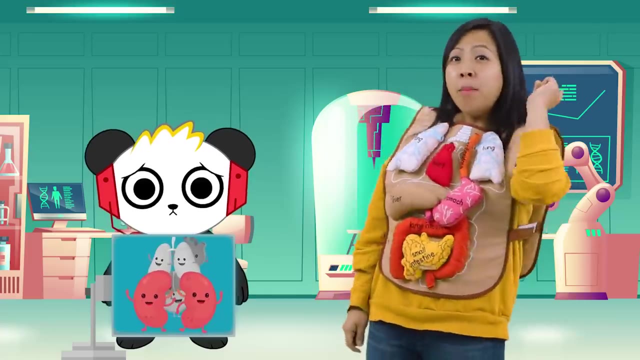 Which organ is next? The kidney will be our last organ, Combo. Come on. Okay, so you should have a pair of kidneys, a right one and a left one. Both of mine are accounted for right. Yes, Combo, Both of your kidneys are there. 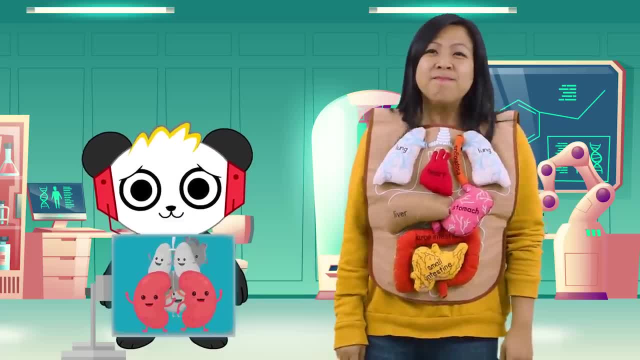 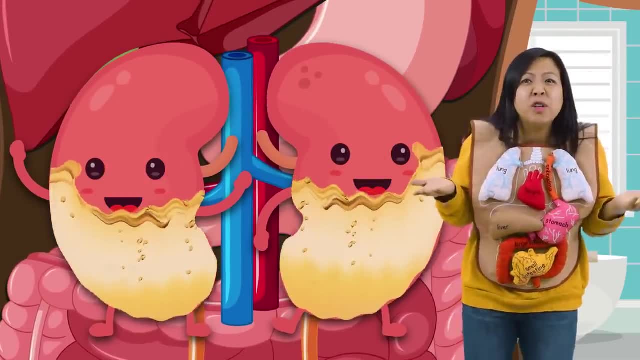 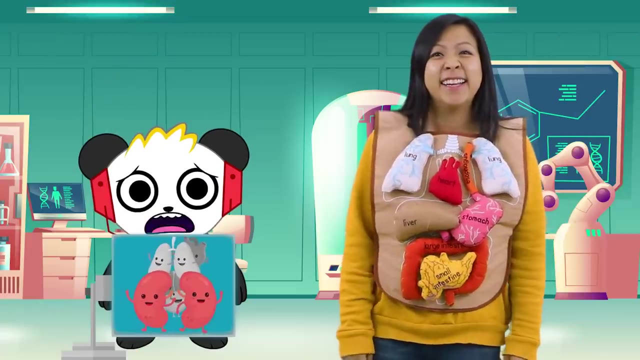 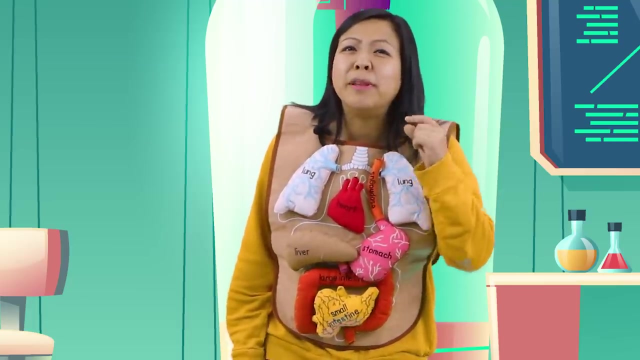 Okay, good, And why do we have them? They balance the body's fluid by removing moving waste and extra fluids from your body in the form of urine. So what if I just drink a giant cup of water before standing here? I'll say you probably really need. 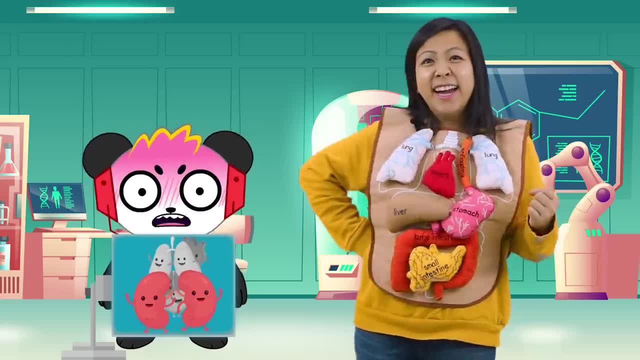 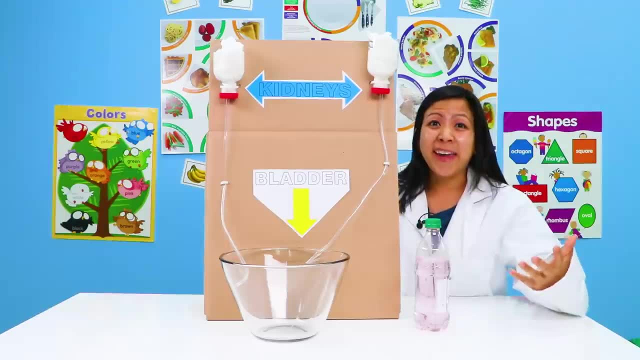 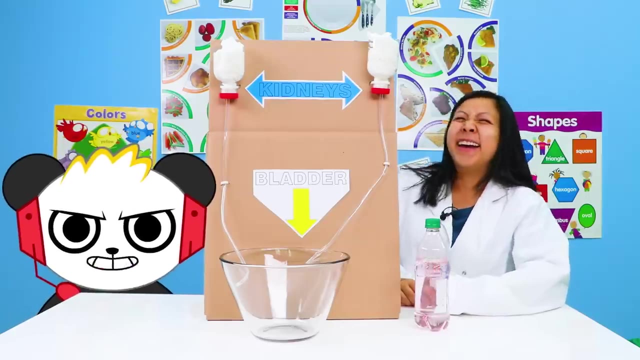 a bathroom break soon. You are absolutely right. I'll meet you at the next experiment. Gotta go, gotta go. Okay, Let me explain to you guys our experiment while we wait for Combo: Wait, I'm here, wait, Okay. so you were saying: 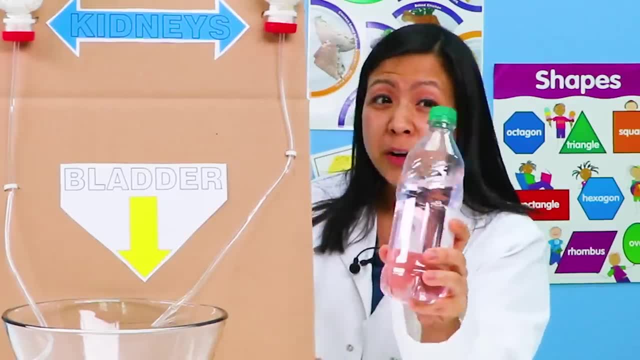 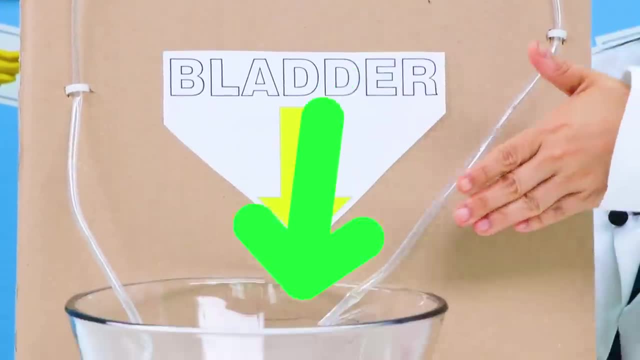 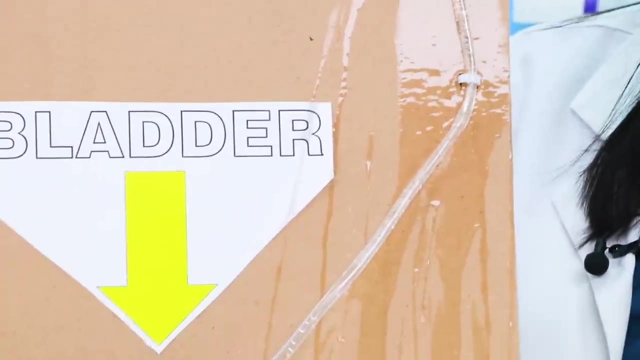 Okay, so we're gonna take our colored water, we're gonna fill up our two kidneys and it will come out of our kidneys into our bladder as urine. Okay, here it goes Into our kidneys, Whee, And into our bladder. 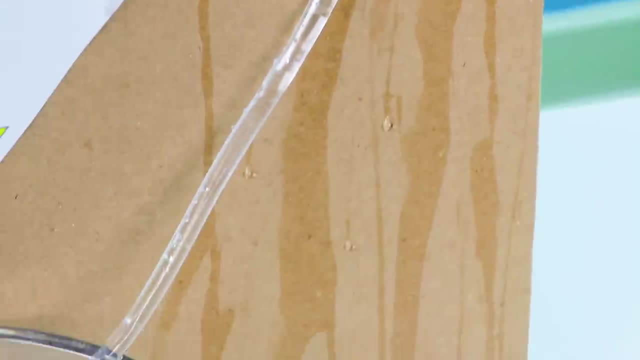 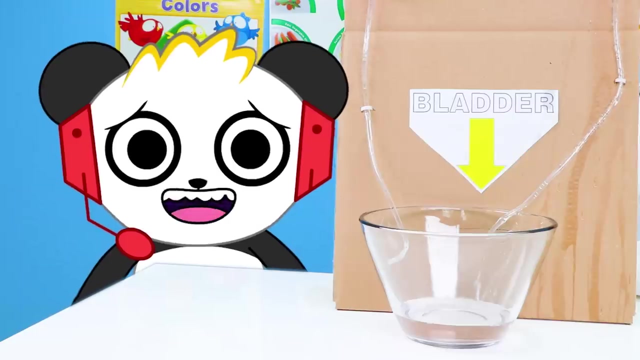 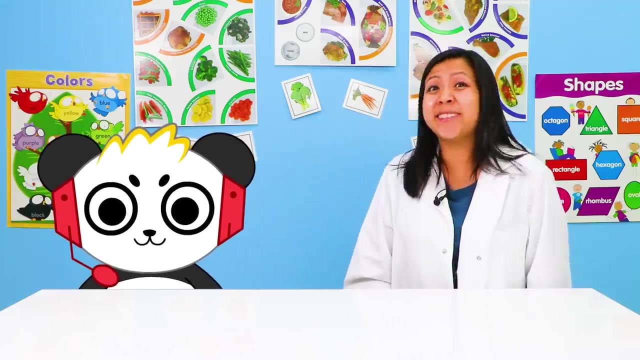 The color was removed, Just like how our kidneys removed waste and our urine fill up the bladder. Wow, I learned so much about my organs. You did a great job, Combo, And you earned your Robux- Oh yeah. How could I forget? 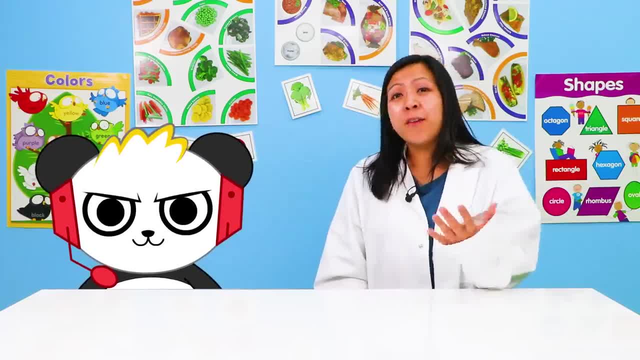 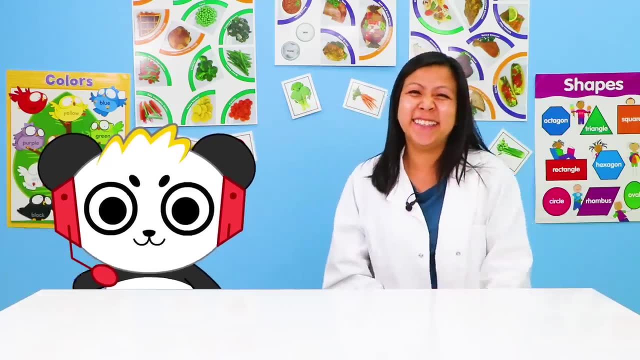 Thanks, Luann, You're welcome, And thank you for helping us learn all about our organs and our body. Okay, Say hi to Ryan. for me I'm gonna go play some Roblox. Okay, thank you, Combo, Have fun. 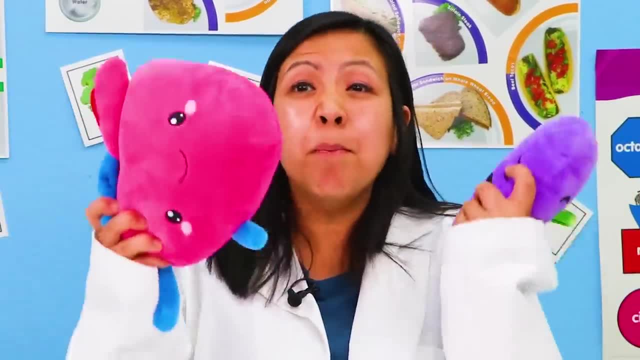 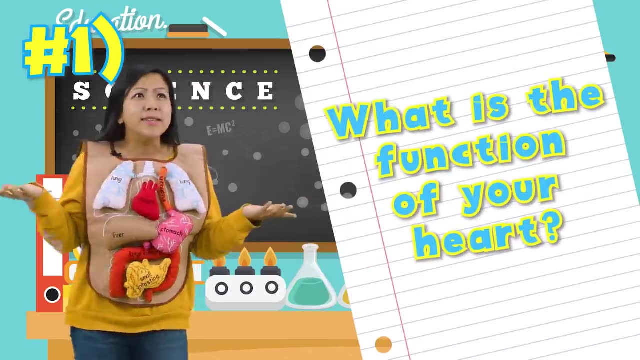 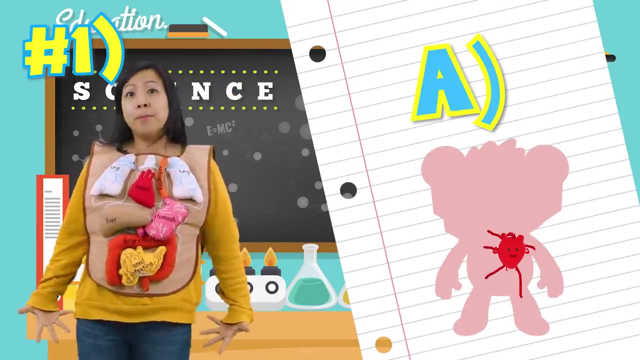 Okay, guys, now let's take a pop quiz to see how much we remember about our organs. Let's go. Question number one: What is the function of your heart? Is it A to pump blood throughout your body, Or is it B to grow fingernails? 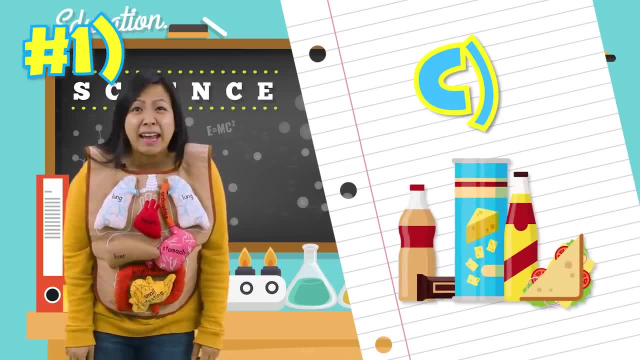 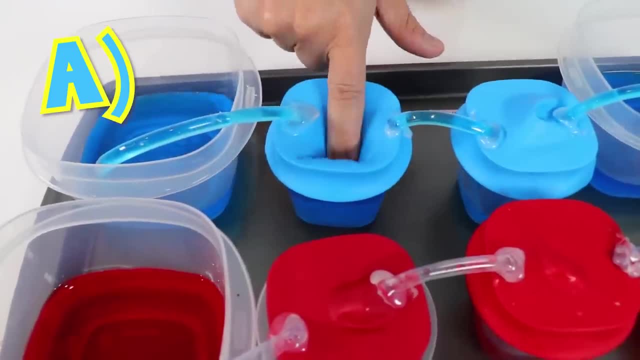 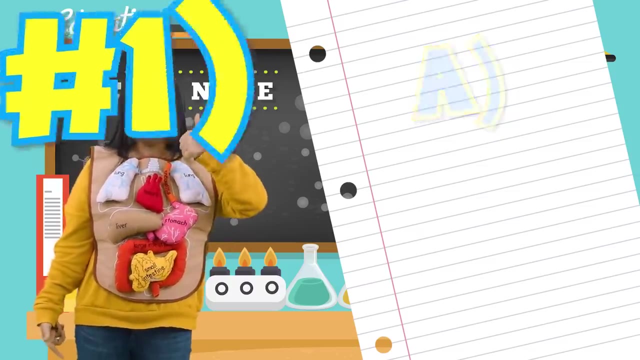 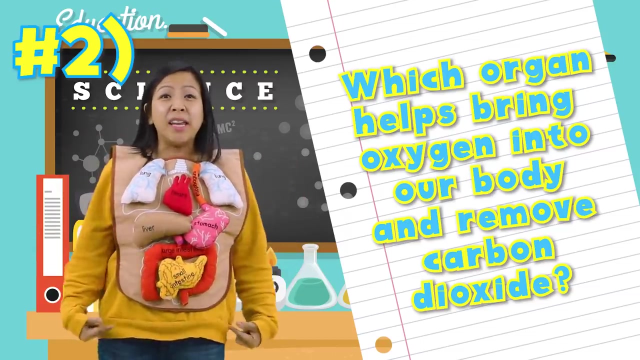 Or is it C to ask for snacks? Did you get the answer? The answer is A. The function of your heart is to pump blood through your body. Good job, heart. Question number two: Which organs help bring oxygen into our body? 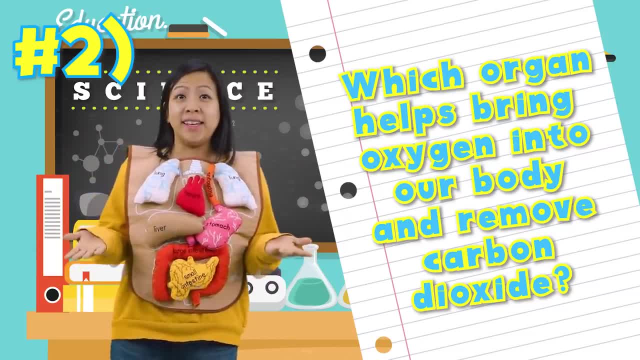 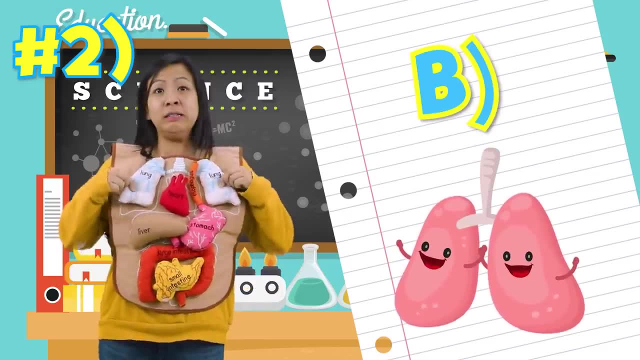 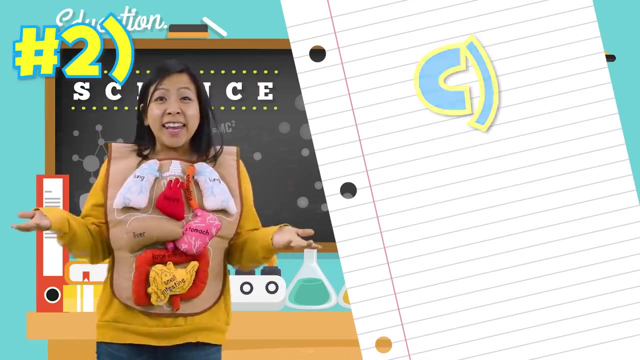 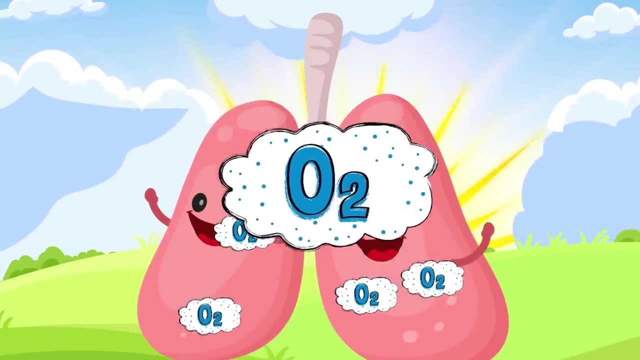 and remove carbon dioxide from our body. Is it A- our toes, Or is it B- our lungs, Or is it C- our knee? Did you get it? The answer is B- lungs, The organs that bring oxygen into our body. 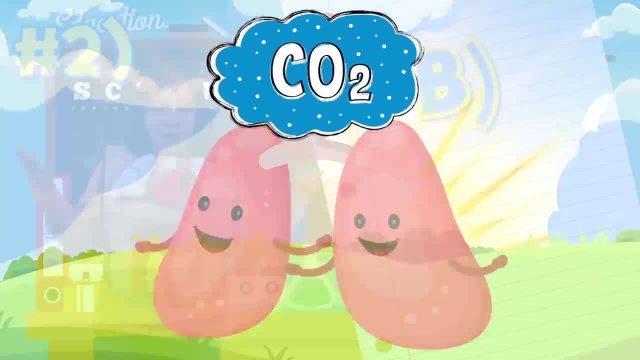 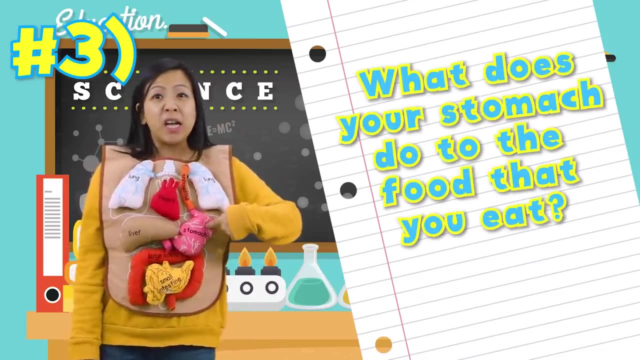 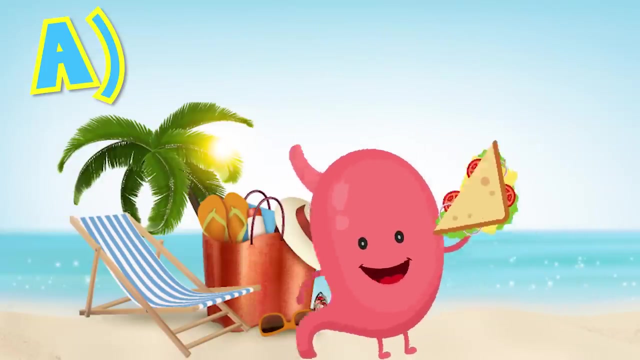 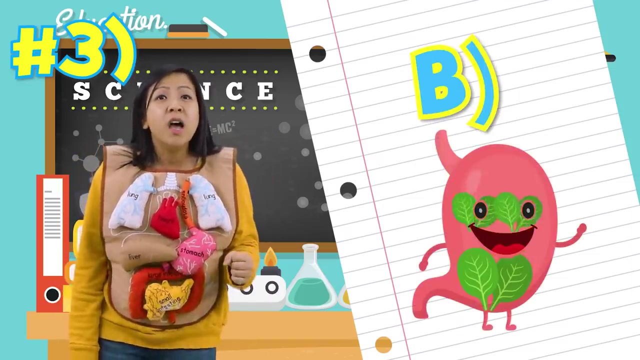 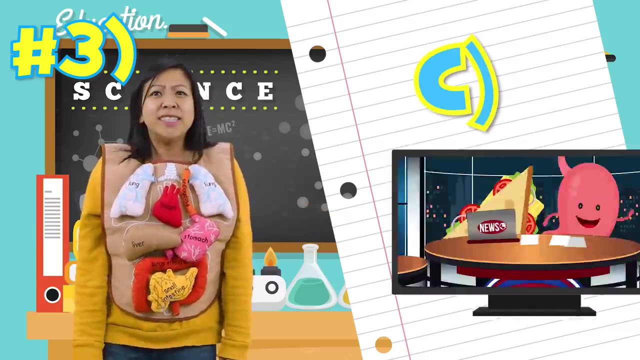 and remove carbon dioxide from our body are lungs. Question number three: What does your stomach do to the food that you eat? Is it A- takes food on vacation, Or is it B- stores, digests and mix food? Or is it C- make it watch TV?